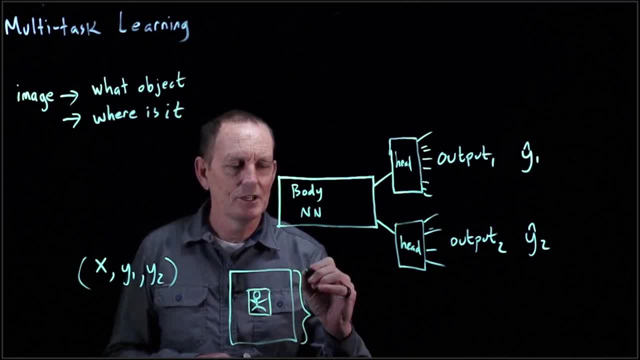 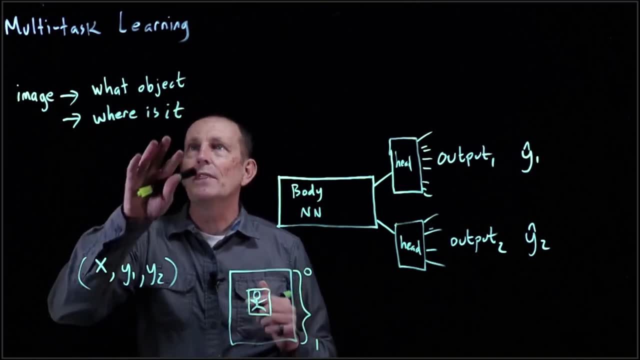 numbers between 0 and 1.. So 0 would mean at the top, 1 would mean at the bottom, half would mean halfway through, nothing more. So you could also have something like that. But y1 is a category and y2 is four. 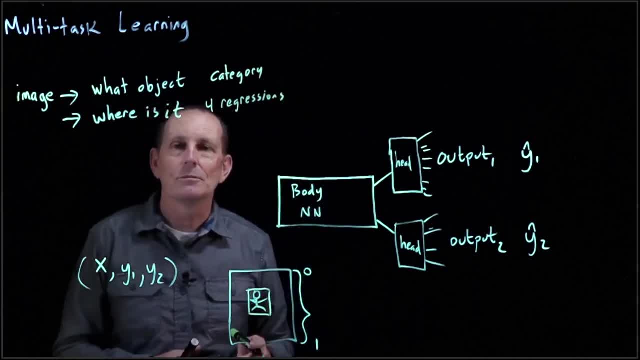 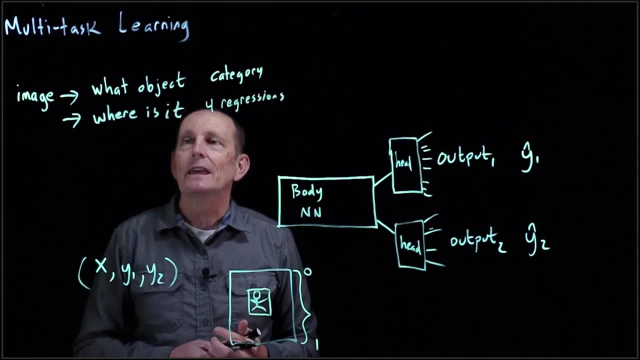 regressions: Top left, bottom right- Maybe it's top left- height and width. whatever we need to do to obtain this bounding box, And what we find is two things. One, if we wanted to make two different neural networks to learn these things. 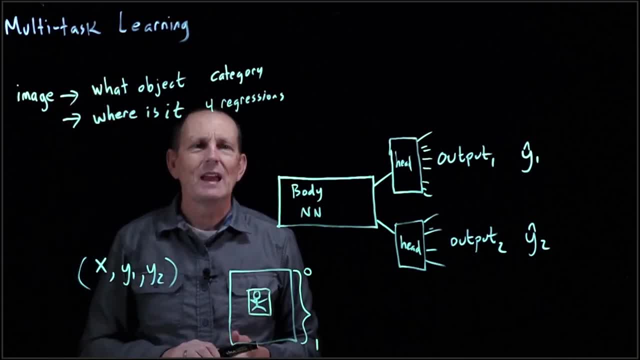 then we're going to get worse performance than if we had one network. to learn both things kind of makes sense, because we have two networks and the totality of weights is going to be much larger than a single network with two heads. The second thing: that's actually somewhat 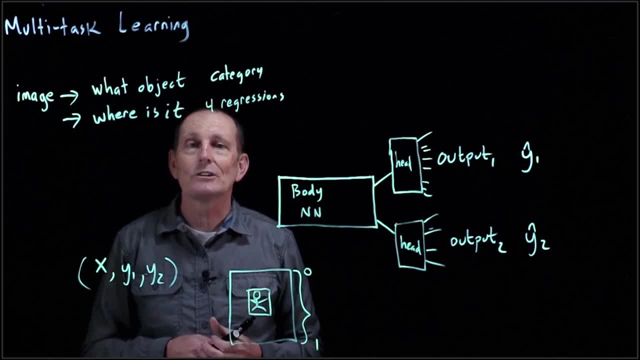 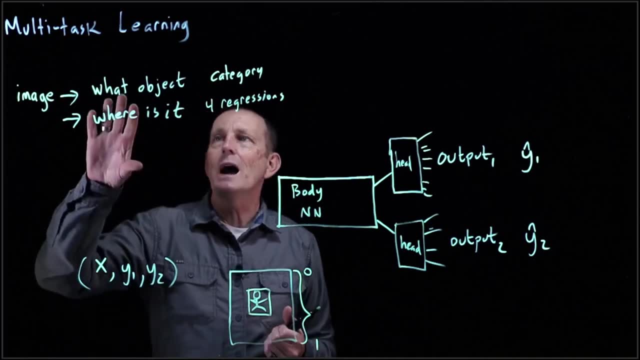 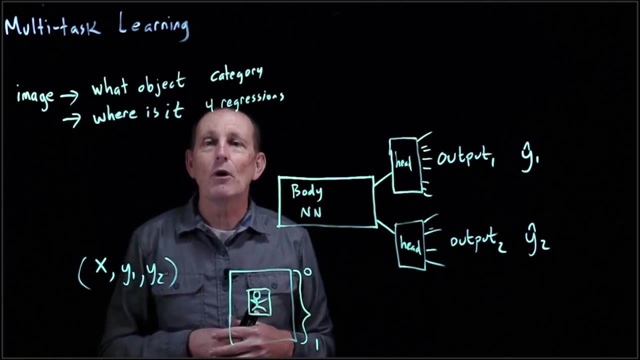 surprising is we get better performance often for trying to learn two tasks than to learn one task, because we've got a beautiful regularization that's coming about. What happens is if you have to learn two tasks, your body needs to be more general. It needs to focus less on. 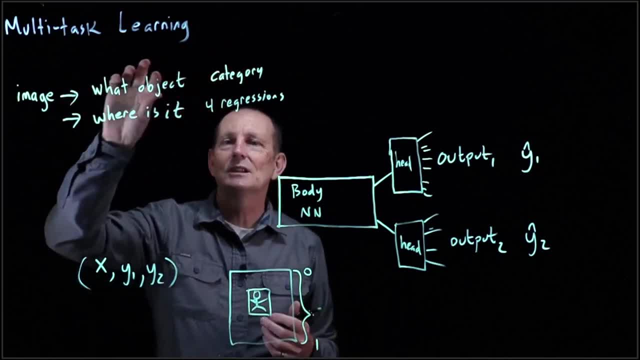 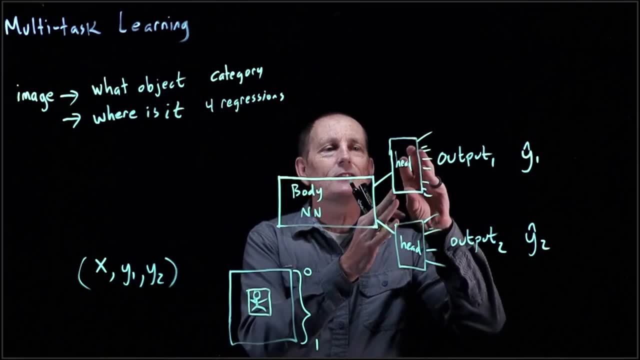 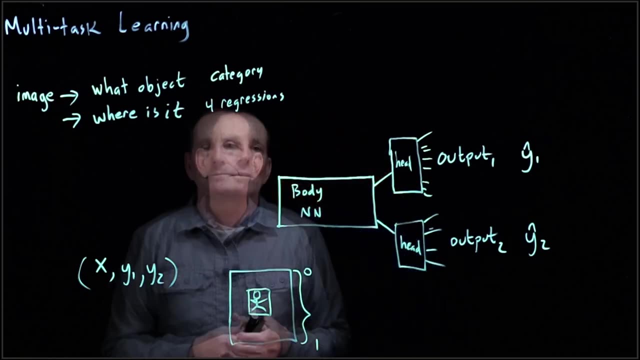 the peculiarities of the particular task and the particular images, and has to be more able to generalize. It has to be a more general body because it's satisfying the needs of not just a single head, to which it's finally attuned, but multiple heads for multiple tasks. 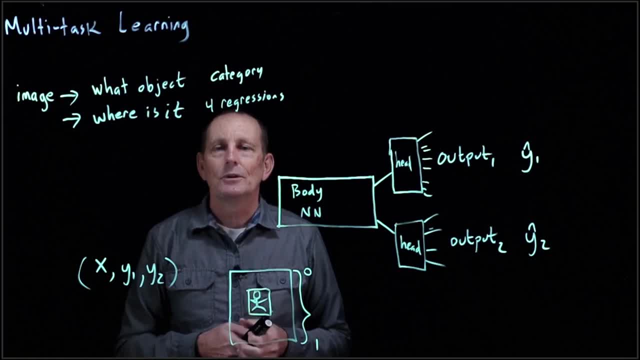 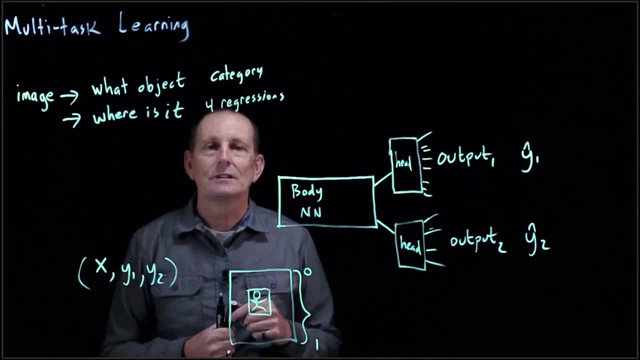 Some examples of this in practice might be, let's say, AlphaGo. They at one point had two networks: One network that was responsible for deciding what the next move is and the second network that was responsible for deciding what the next move is and the second network. 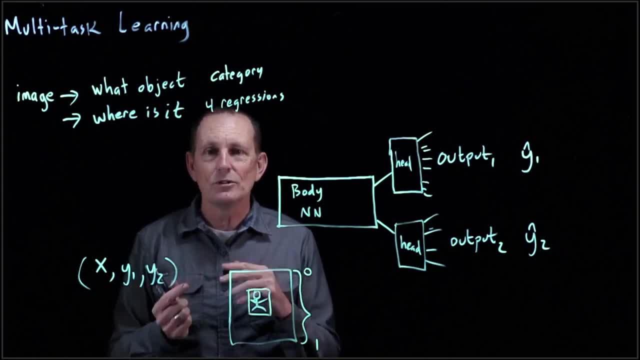 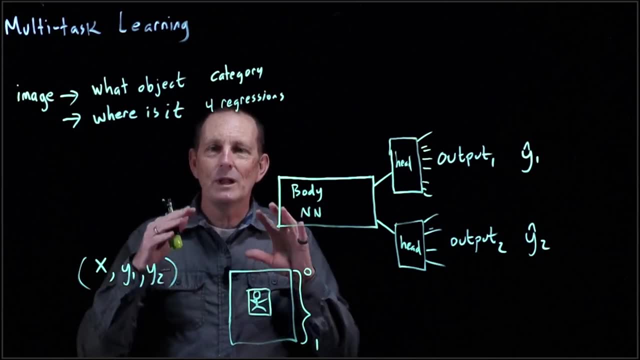 was responsible for predicting, at this point in time, who's most likely to win white or black. In later versions of AlphaGo, they went ahead and merged those two networks into a single network, and that single network had two different heads. One head would decide. 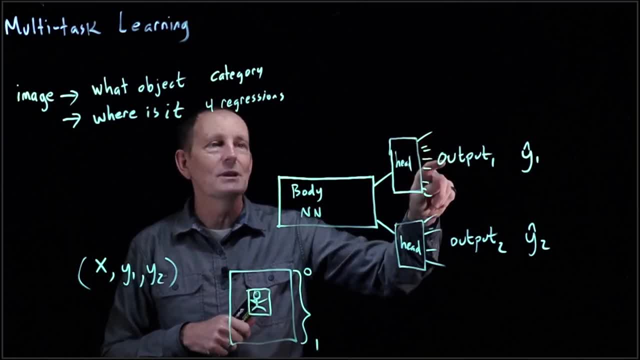 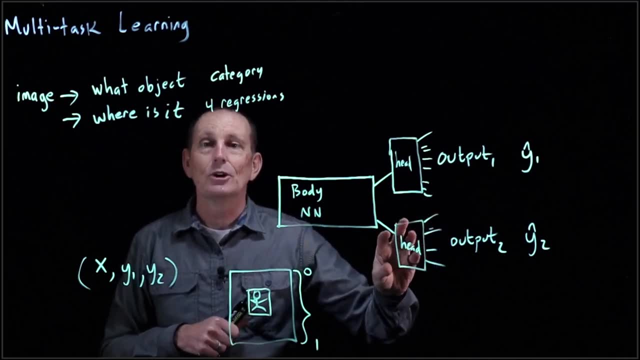 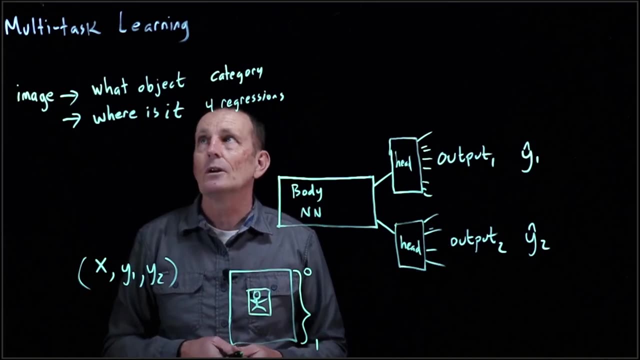 what's the best action to take, and that was just a big softmax of all possible moves. and then the second head was a predictor as to who was likely to win, and that was just a single sigmoid output. But that's kind of how multitask works. in terms of adding these new heads, We have talked. 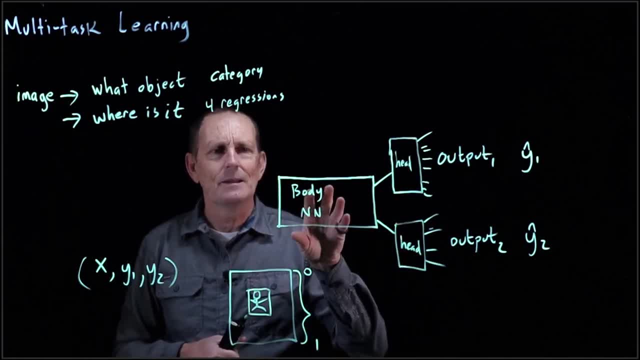 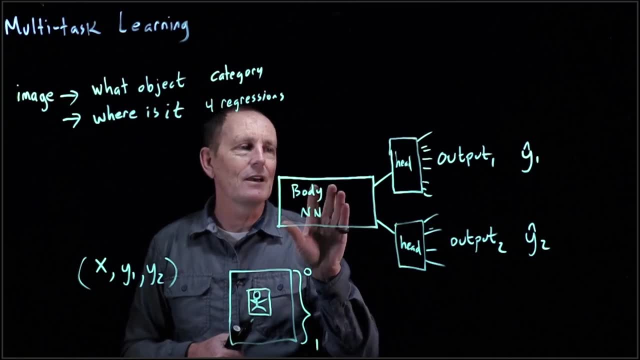 earlier about multitask running, but haven't talked in any particular detail about how actually we make the multitask working. and the way we make it work is we have this single neural network and then we have just these different outputs on top. When we look at 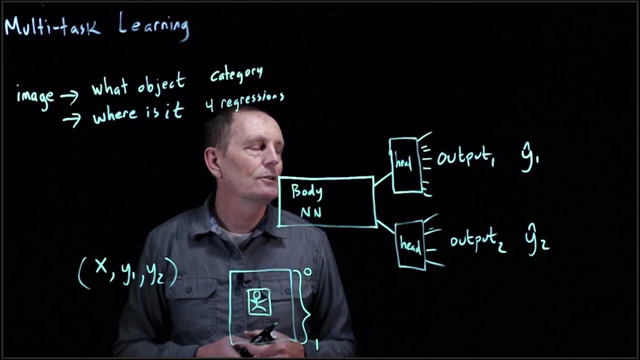 the separate heads, you're gonna see you have your single layer, then you have your single neural network. When you look at the separate heads, you will see that all the different heads here right. What we can really have is: so we've got these outputs. 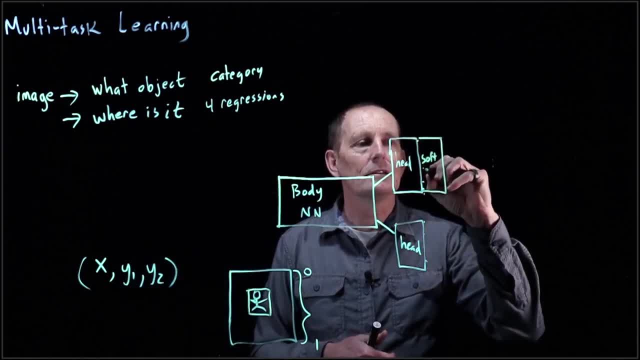 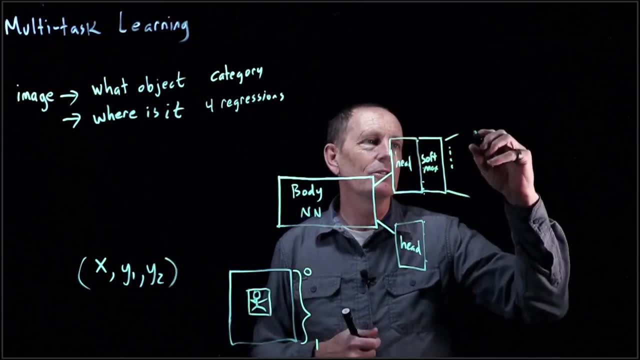 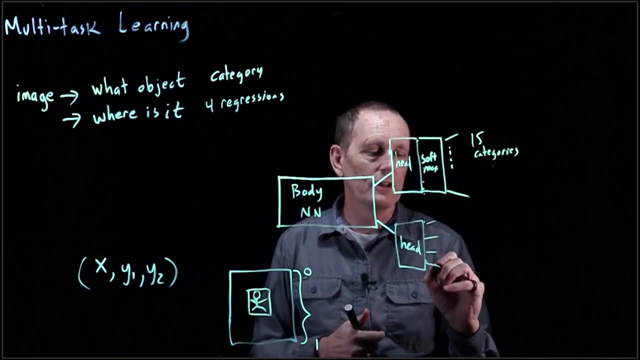 Let's say, here we have softmax with some number of outputs, And here let's say: it's this example here. So we've got I don't know 15 categories, And here we've got a bounding box, so we've got four values coming out. 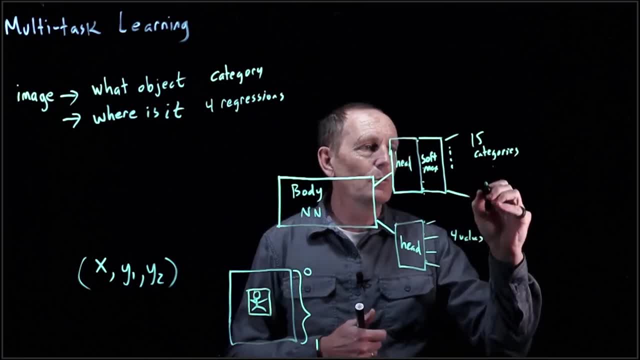 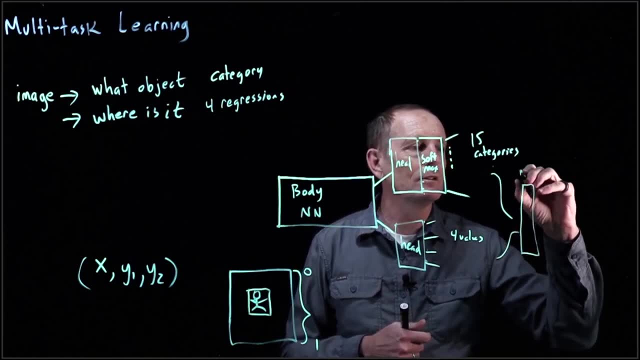 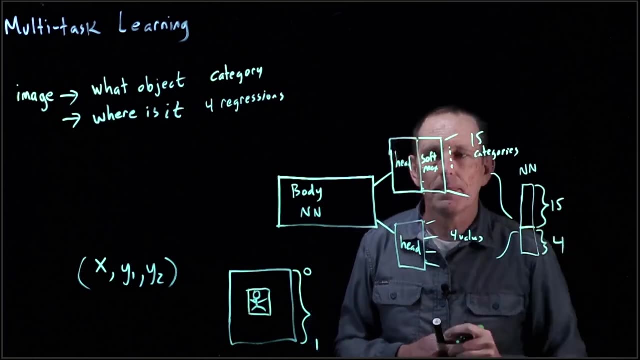 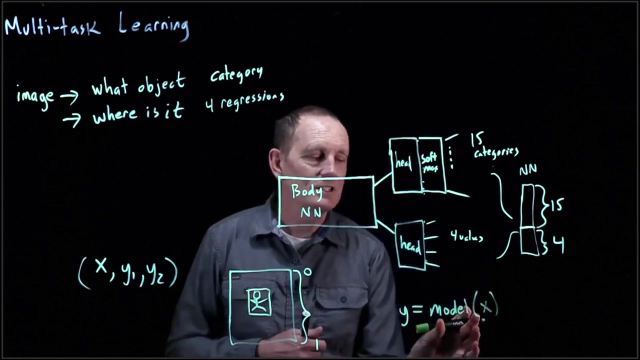 We can actually merge these together. So the final output, the last layer of our neural network, is really 15 categories plus four values, And what that allows us to do is actually say something you know: y equals model of x, That is, if this is running the neural network. 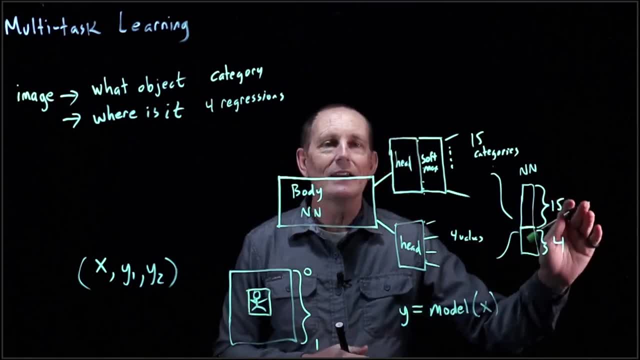 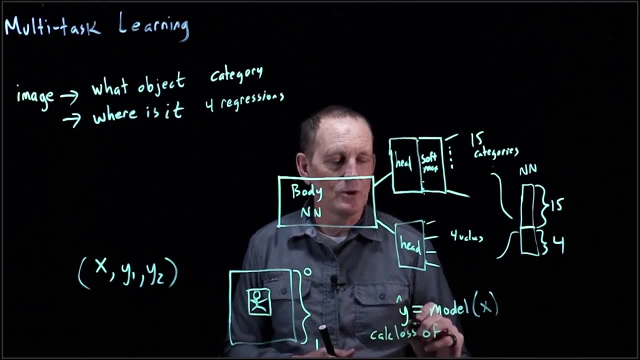 we can feed in and get out a single y, And this single y would have 19 values, And then what we can go ahead and do is calculate the loss. This, of course, is y hat, The loss of y1 and the first 15 values of y hat. 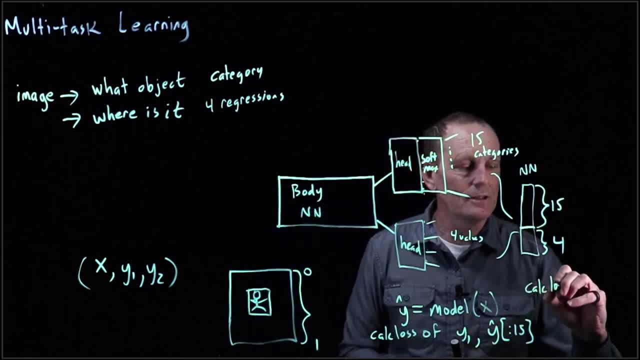 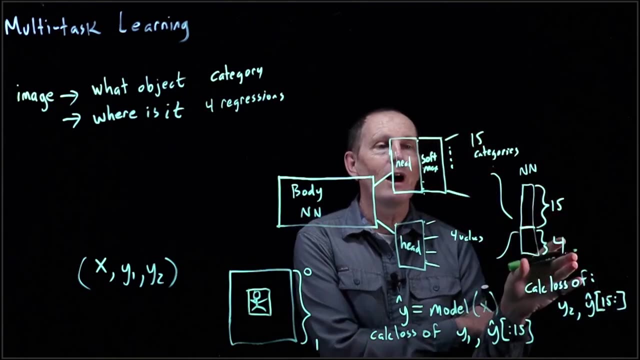 And then also calculate the loss of y2 and y1. And then we can put 15 on. That is 15,, 16,, 17, and 18.. So we're coming out with a single y hat that we can then break back down into the various y hat1 and y hat2.. 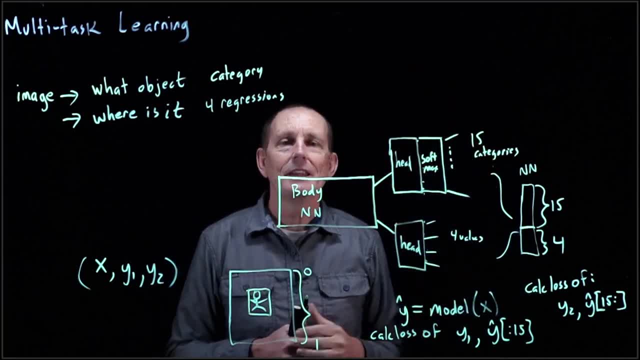 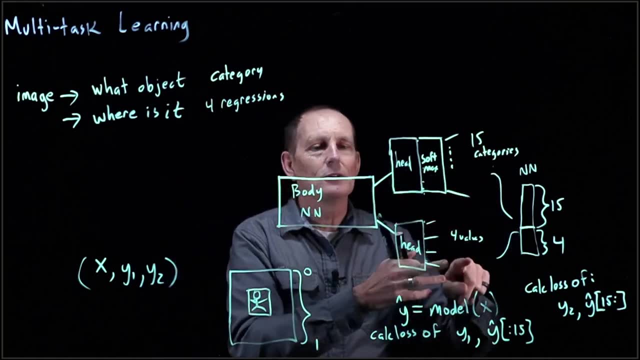 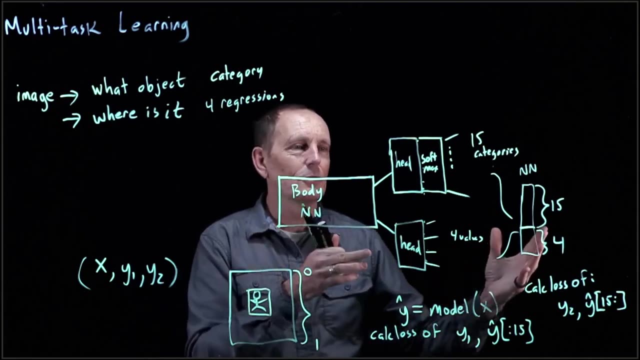 My previous picture actually showed completely separate heads And in that case it was a little unclear how you would take an x and go ahead and feed it out to the y1 and the y2 without going through the body twice. And we certainly don't want to do that, because when we do our back propagation